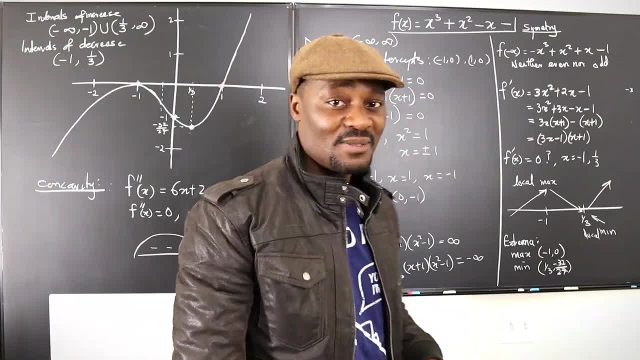 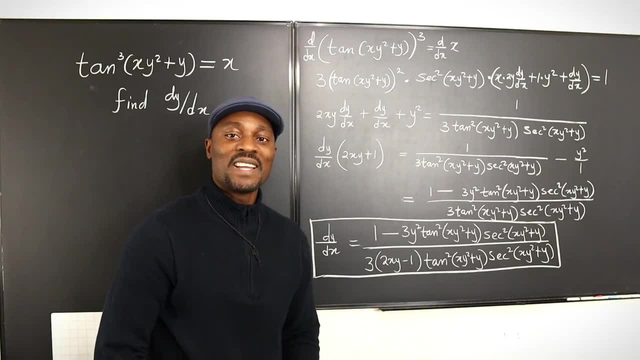 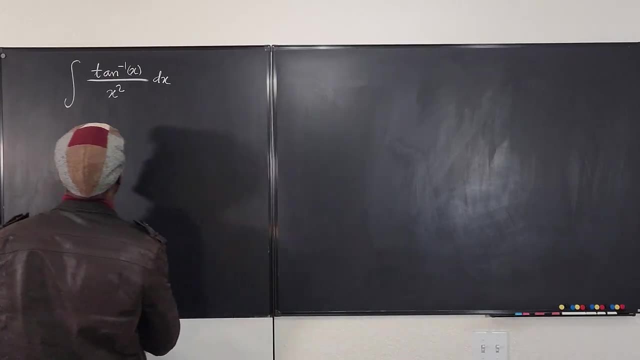 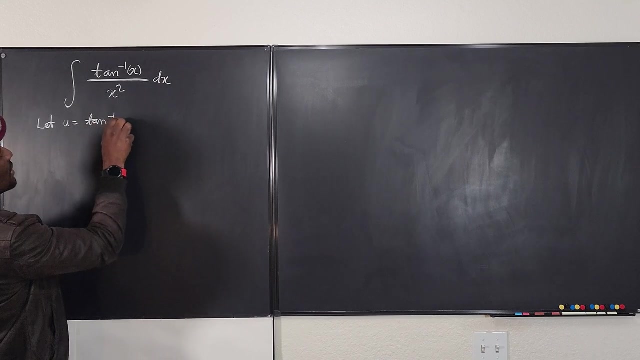 get from that. So we're going to write u as r-tan x and see what we get. Let's say, let u be equal to the r-tan of x dx. What will be the derivative? We know the derivative of r-tan of x because 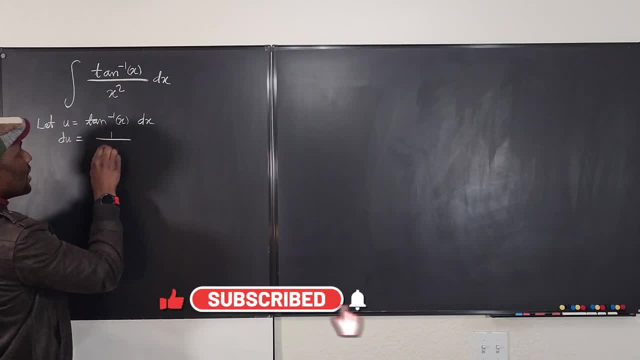 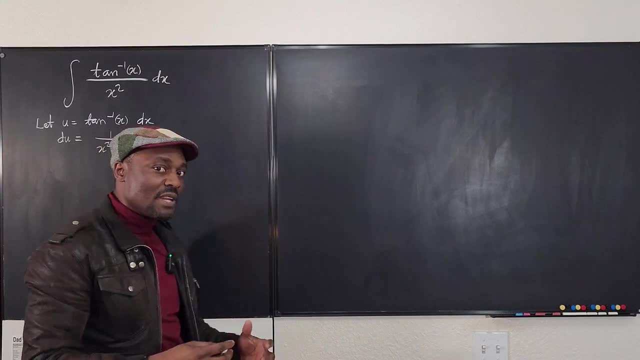 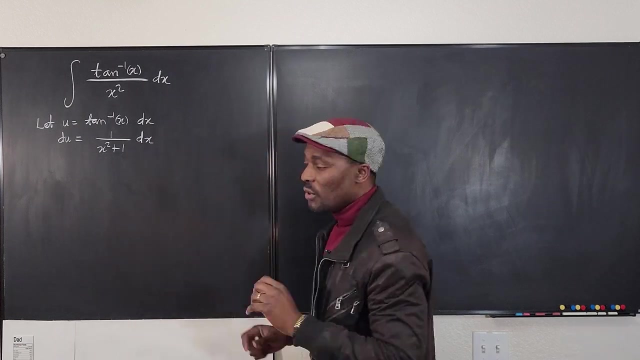 that's why we chose it. It's going to be 1 over x squared plus 1.. We've done this before. Yeah, you're supposed to know this. okay, So the differential now is 1 over x squared plus 1 dx. But remember, usually when we do a u-substitution, it's 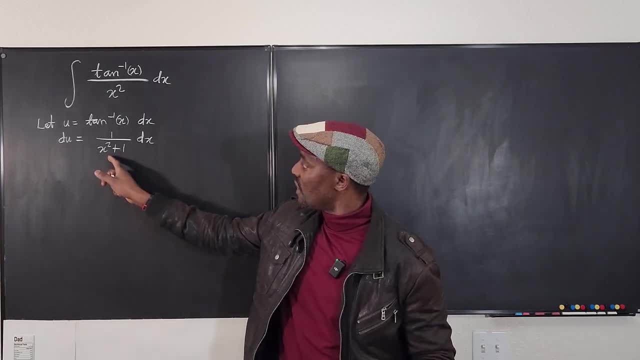 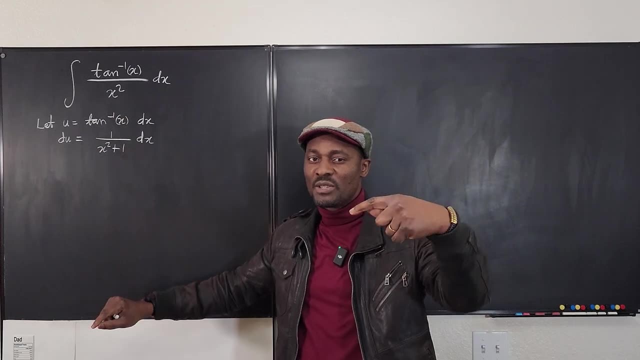 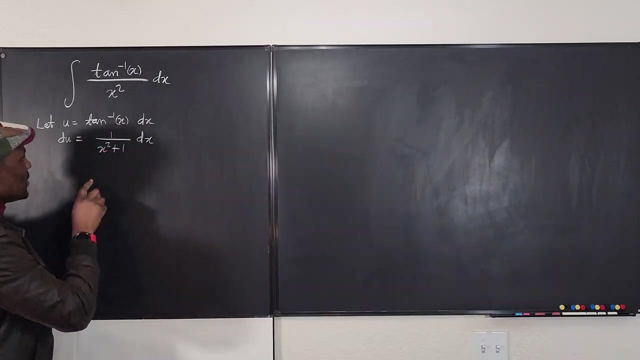 because you want to get rid of x completely. but it appears that our derivative still has x squared plus 1, and we want to get rid of this. But remember the original substitution. We said that u is r-tan of x. Let's go play with this a little. What do you think we're? 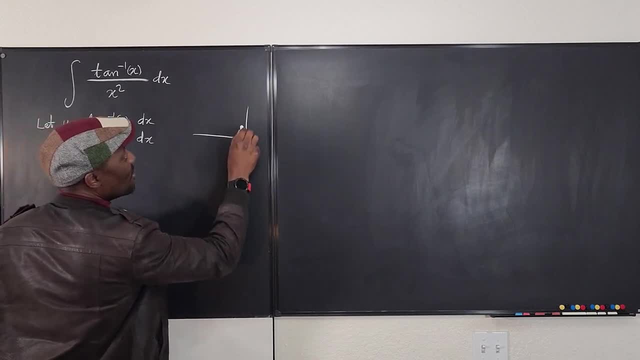 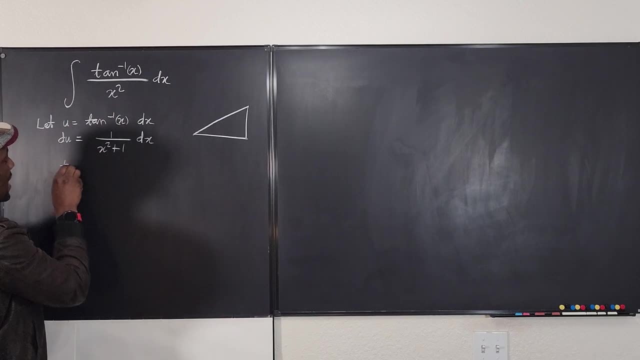 going to get. Let's do this triangle. There's going to be an amazing discovery, because if r-tan of x is u, it simply means that the tan of u, if we take the tan of both sides, equals the tan of r-tan of x. Okay, 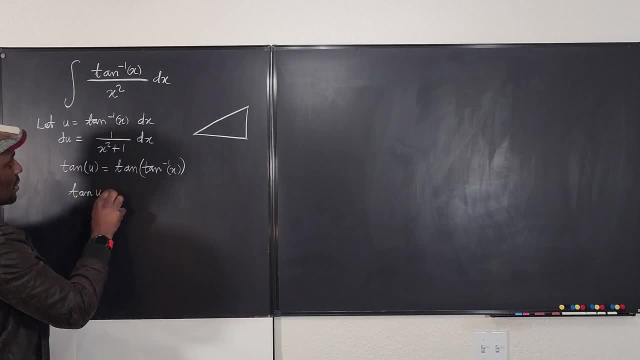 Remember that this simply means that tan of u will be equal to x. Oh, so x is tan u, So it looks like x squared plus 1.. plus one can be written as tan squared u. or we can say: tan squared of u is equal to x squared. 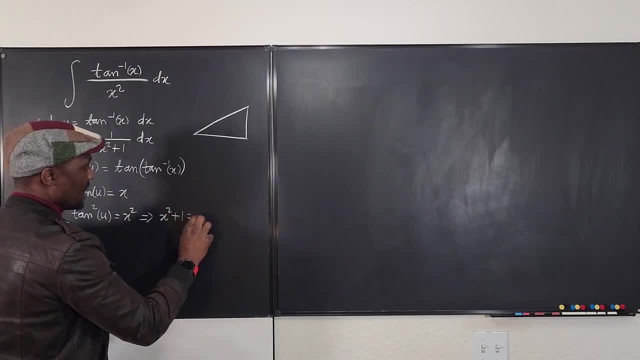 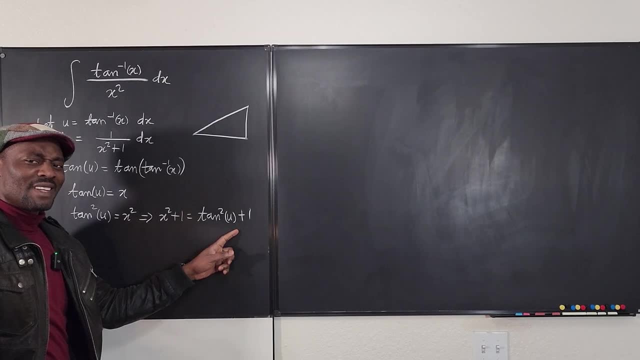 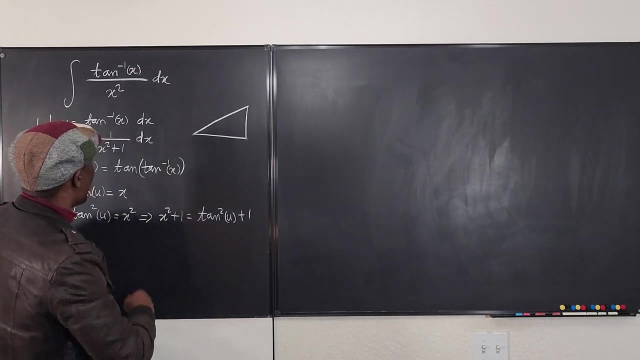 which implies that x squared plus one is equal to tan squared u plus one. Do we know what tan squared u plus one is? Yeah, that's secant squared u, So it looks like the problem is gradually getting solved. Okay, so x plus plus x squared plus one is going to be secant squared u and. 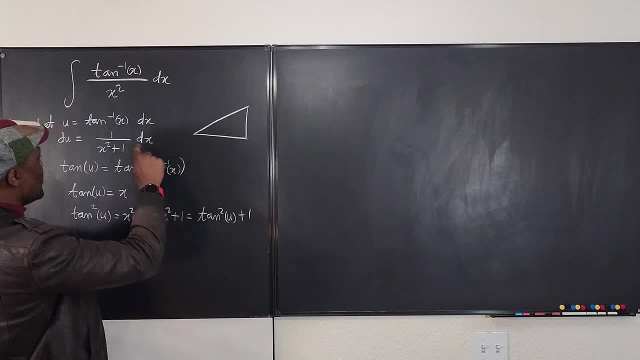 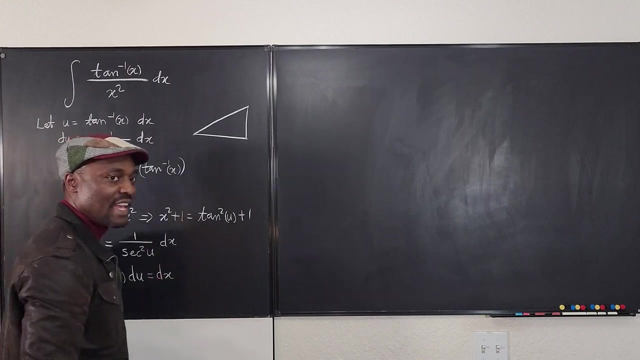 let's go back to this derivative, So we can say: therefore, du will be equal to one over secant squared u- dx. So if you multiply both sides by secant squared, we're going to have secant squared u, du is equal to dx. Okay, see, we've gotten rid of everything that is called x at this point, because we know what. 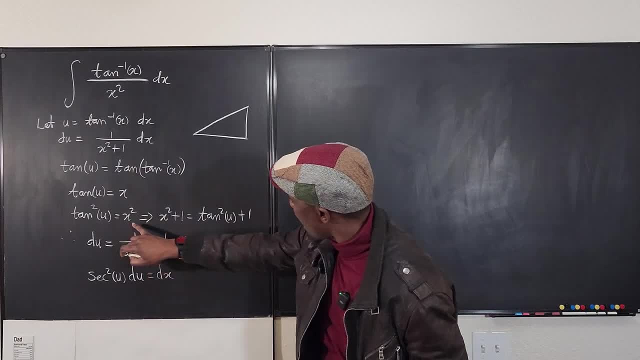 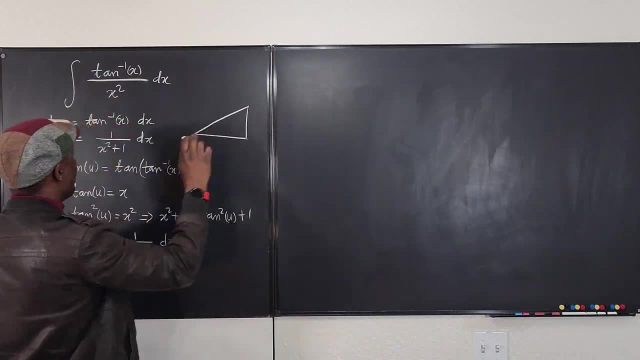 x squared is in terms of u. What is x squared? x squared is tan squared u, and we also know that this is now replaced by u, and let's do this here. We know that x is tan u If tan of u is x, that's. 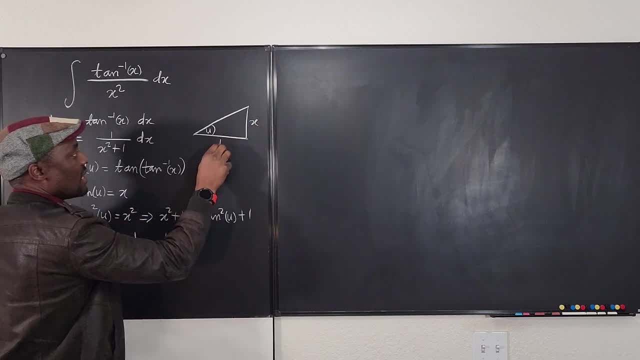 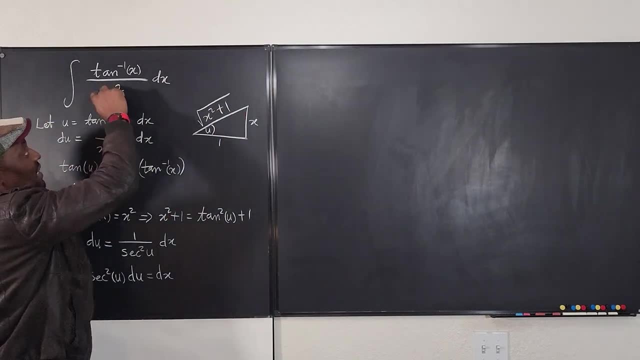 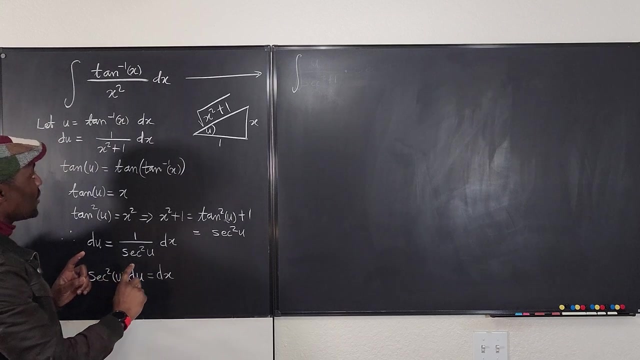 x tangent is opposite over adjacent, So this is going to be the square root of x, squared plus one. We've got all the ingredients that we need, So let's go back here and write this integral, So this integral here, So the integral of what do we have? We have, this is going to be u. 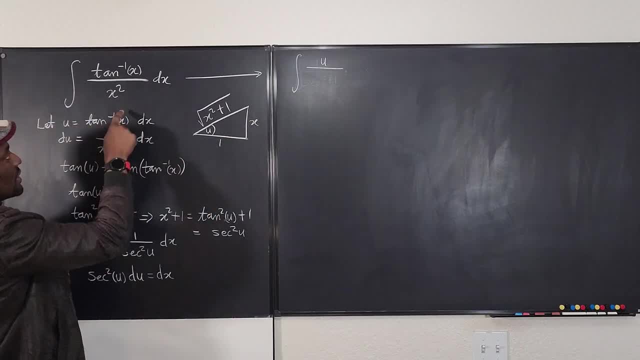 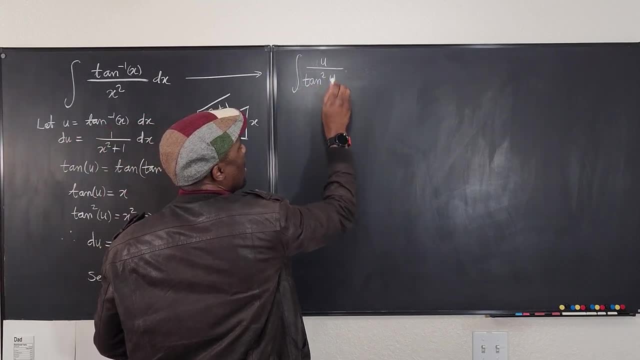 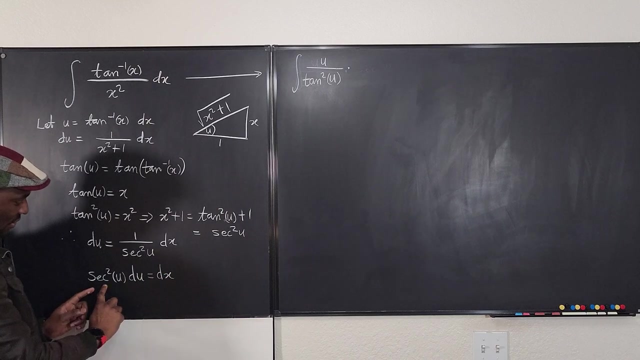 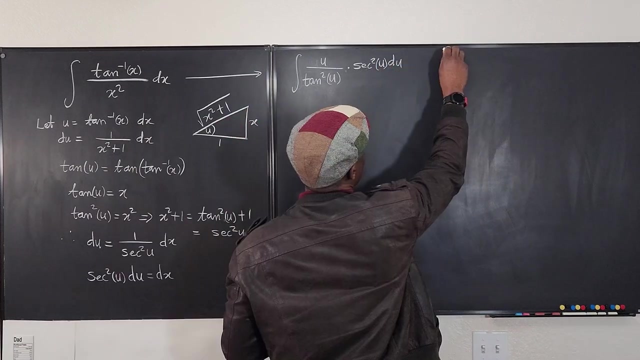 because that was the substitution. u is r tan of x, and then x squared is tan squared u, That's tan squared of u, and then we need to replace dx, which we found. dx is secant squared u du, So that's secant squared u du. Nice, Let me make this easier. Is that a? 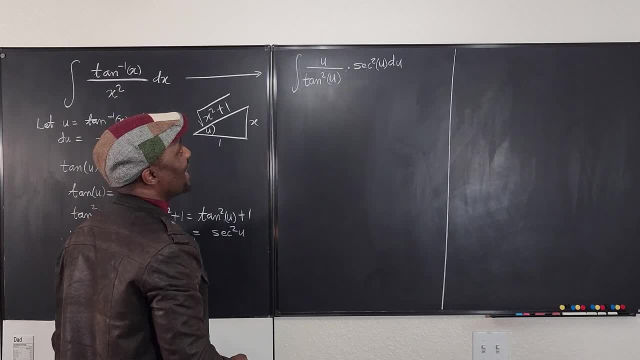 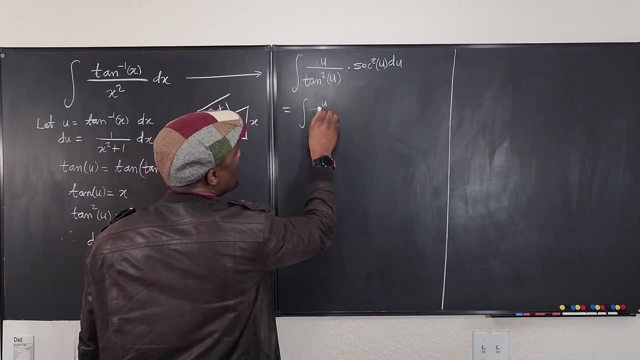 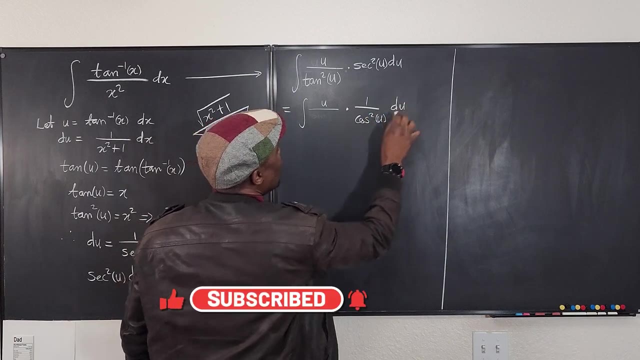 straight line. I don't know, It looks terrible though. Okay. so this is the same thing as the integral of u over is one over cosine squared And this is going to be tan squared. u Okay, Makes life a lot easier. This is the integral. 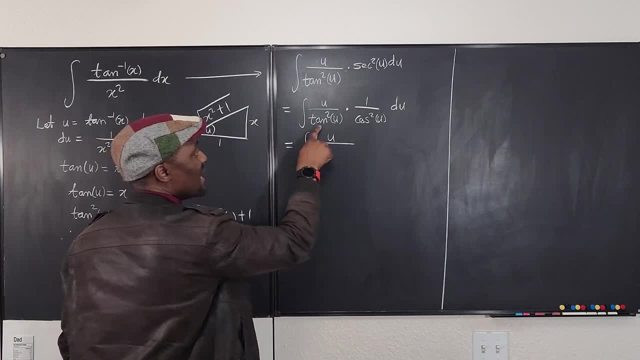 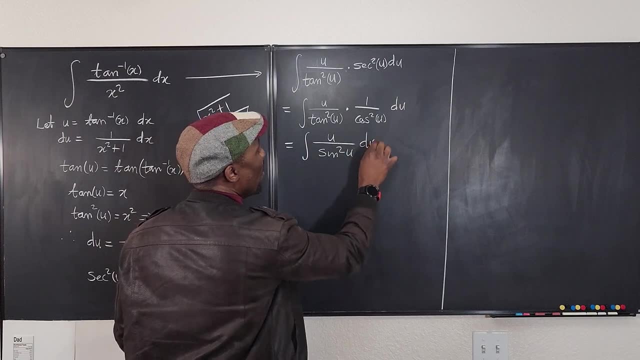 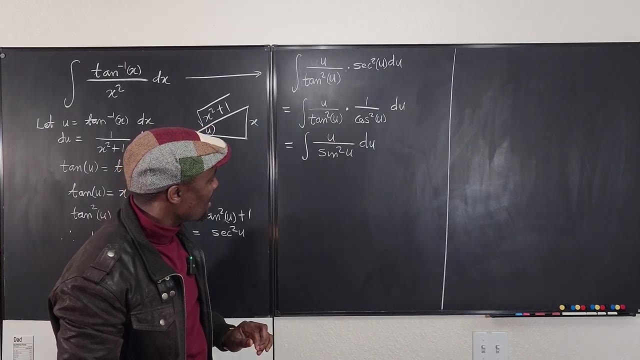 of u over. Remember that tan squared tan times, cosine is sine, So this is going to be sine squared u. Oh, now this integral is beginning to look like something we can do. So here, what do we have? This is, I don't know what to do. u substitution is not going to work either, or? 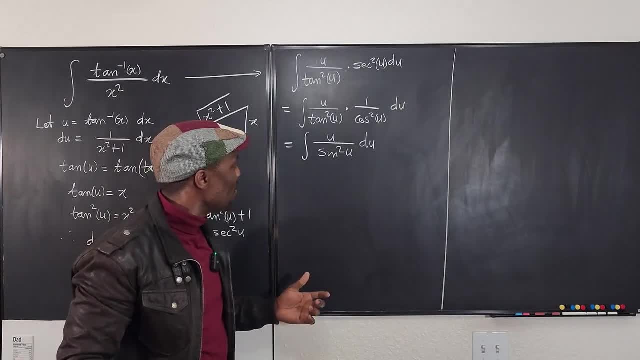 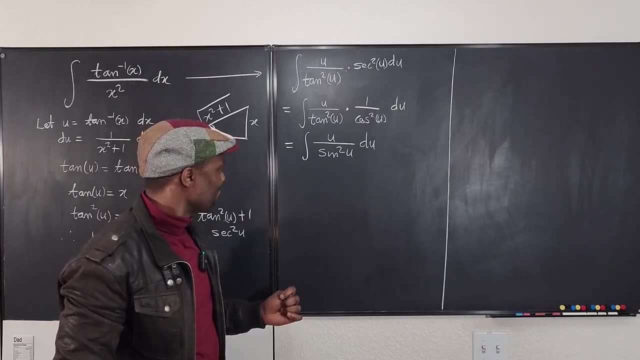 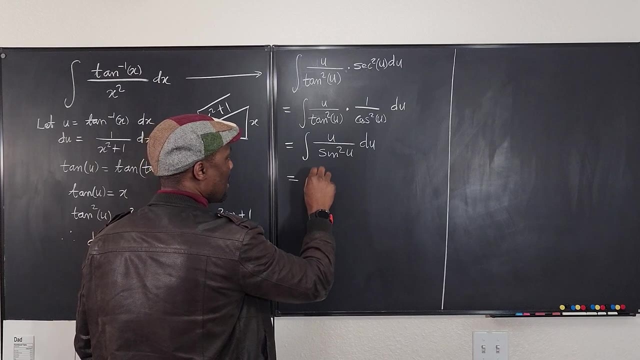 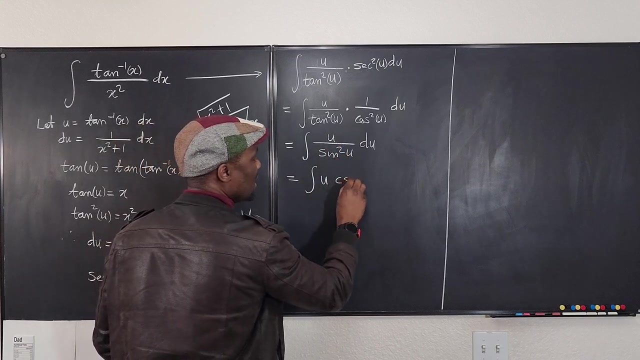 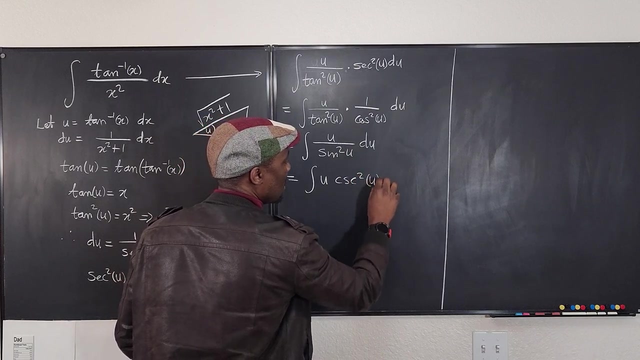 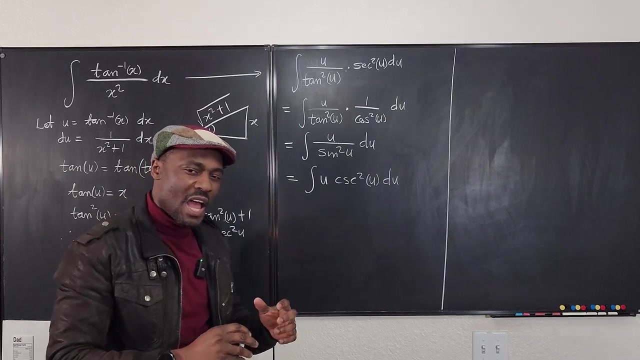 we've used u already, so t substitution won't work. I might have to do integration by parts, So let's rewrite this as if it were the integral of u times one over sine squared theta is: cosecant sine squared u will be cosecant squared u du. Okay, Which one should we choose as our dv? Which one is du? You know this can be. 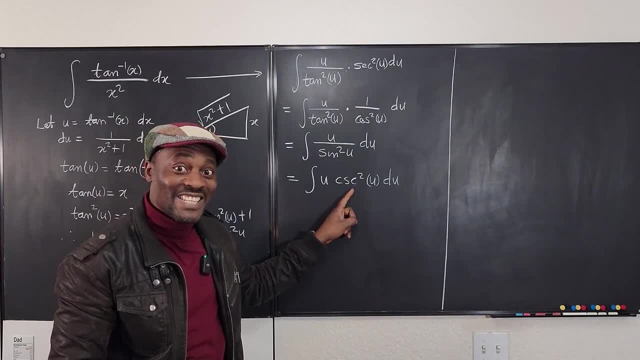 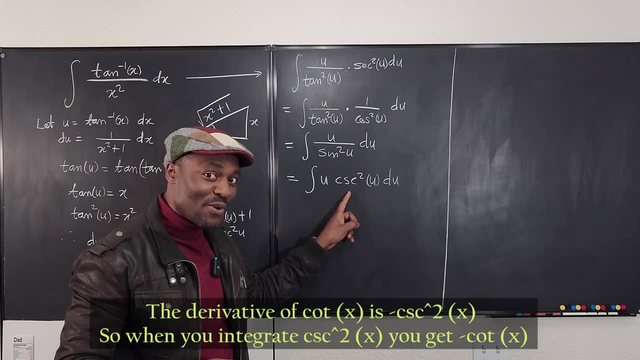 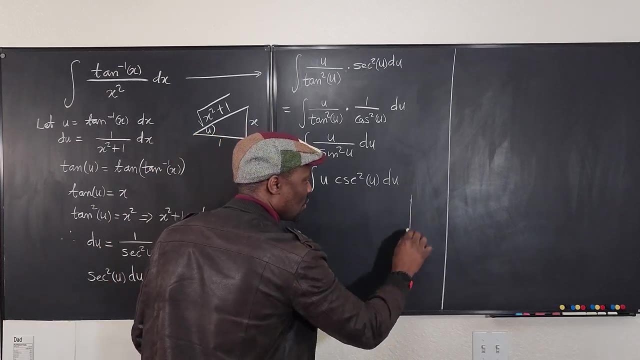 easily differentiated and this can be easily integrated. Remember that the derivative of cotangent is negative cosecant, So the integral of cosecant is negative cotangent. So that's the choice we should make. I'm going to use the table. Okay, So I'm going to choose what to differentiate and what to integrate This. so I'm going to write. 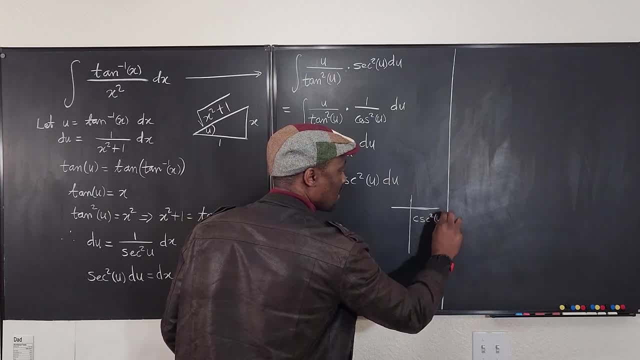 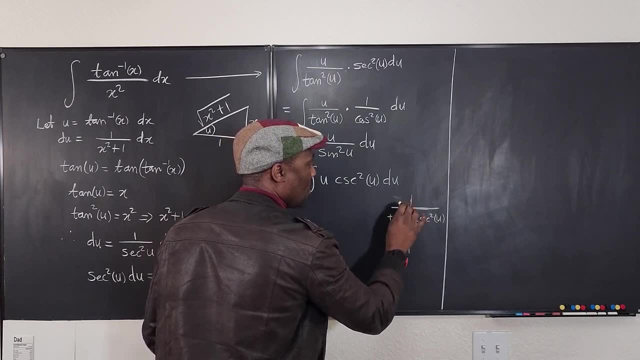 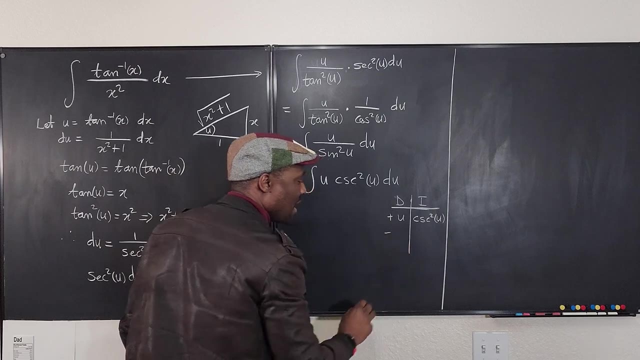 cosecant squared u and I am going to differentiate this u with the plus. So I differentiate or I'm going to call this my u. I don't want to use u. I'm going to call this differentiate and integrate. I call this the di method, and then I'm going to have 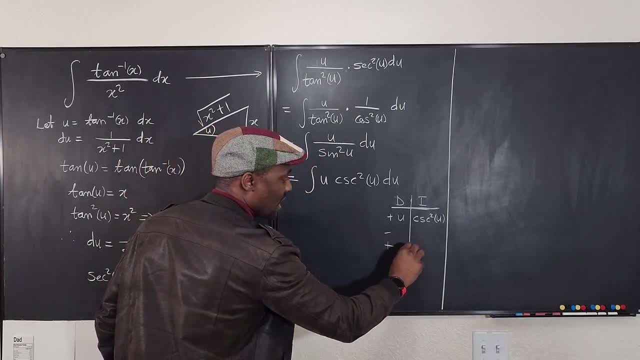 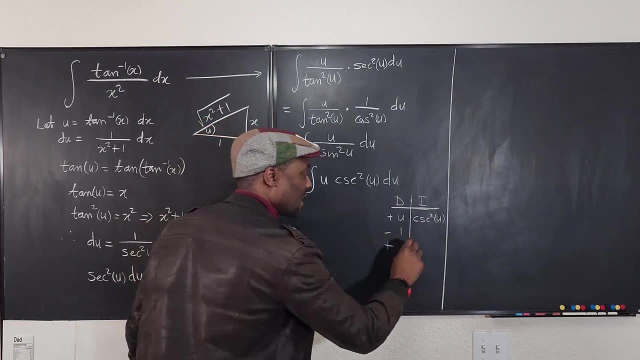 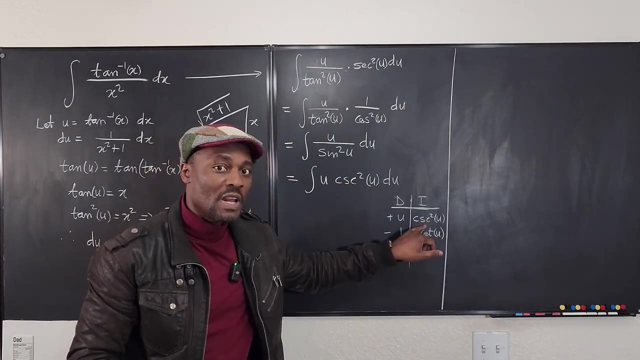 my minus sign here and then plus, we'll see how far we need to go. What is the derivative of u? it's one. what is the integral of cosecant? it's negative cotangent. so this is the only part that might be tough for anyone, because you don't recall that this, this is the derivative of this. so when 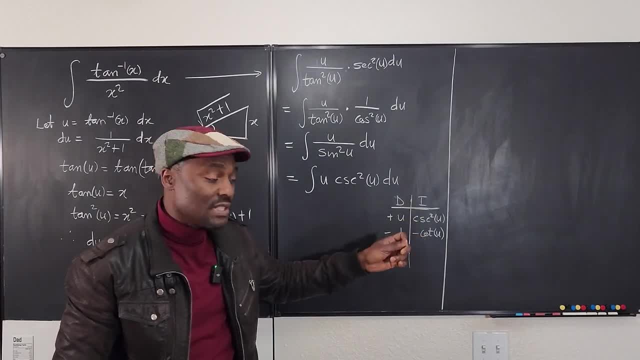 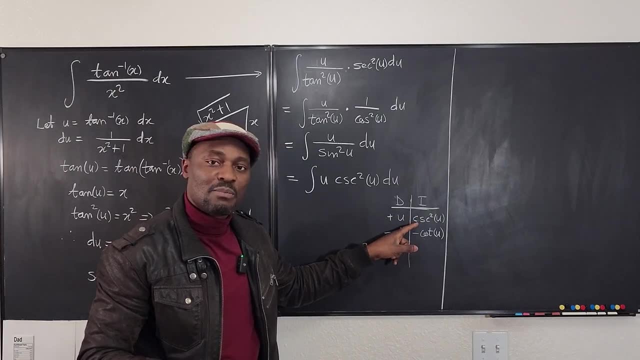 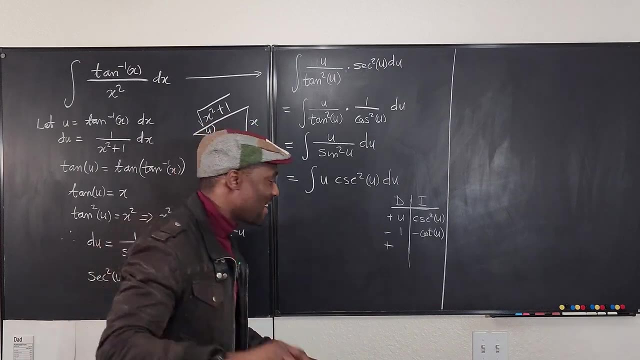 you integrate this, you get the negative of this. actually, it's the negative of each other because they are complement of each other. usually always look out for negative signs when you see the prefix co, cotangent, cosine, cosecant, will always come with a negative. okay, remember that. okay, so. 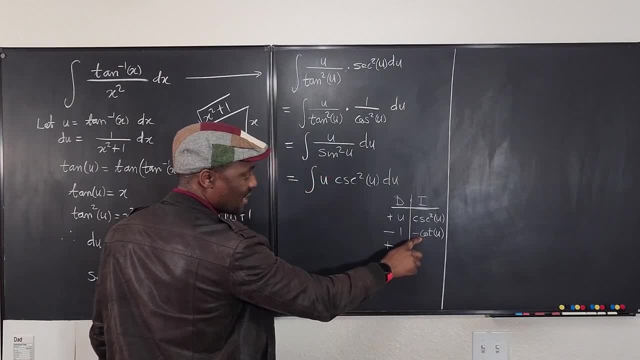 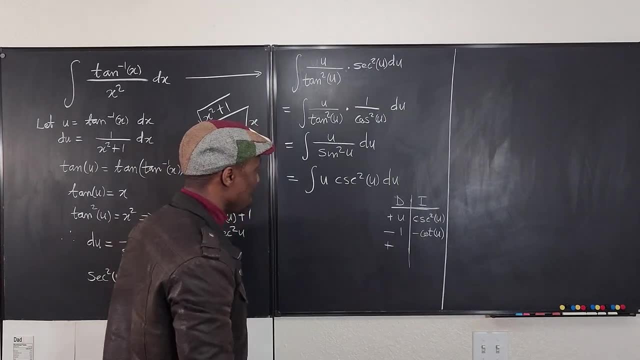 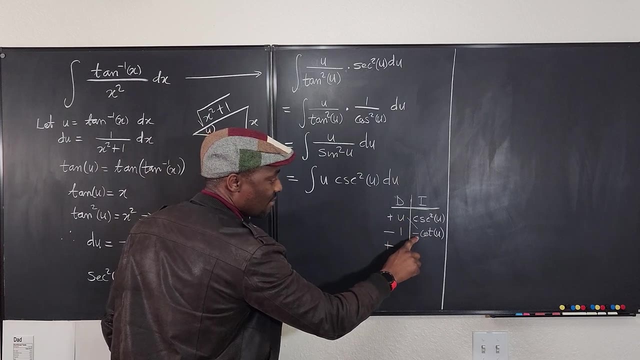 this is minus and i think this is fine. we can integrate this. so usually you stop when you know you can integrate this one. okay, so i'm going to stop here, and it means this is what we have. our integral is going to be this, which is negative u. so this is negative u. 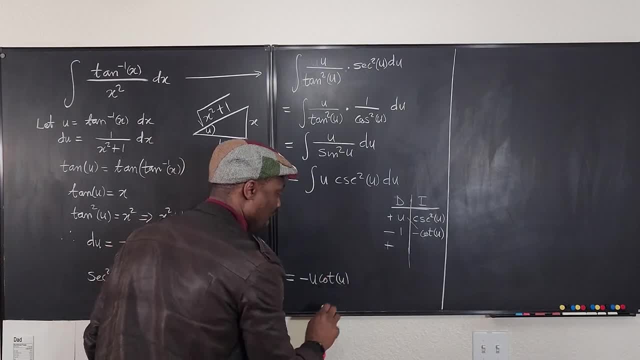 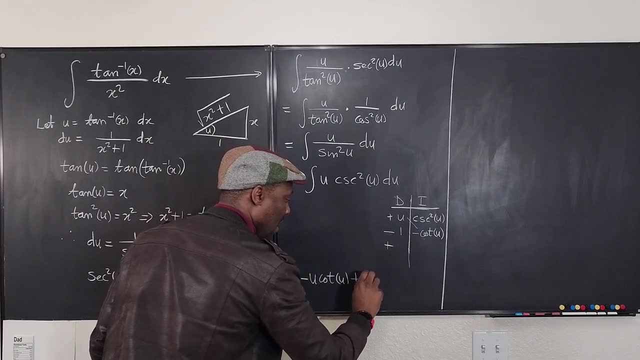 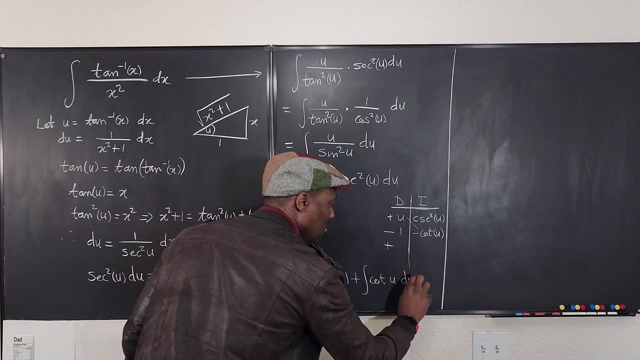 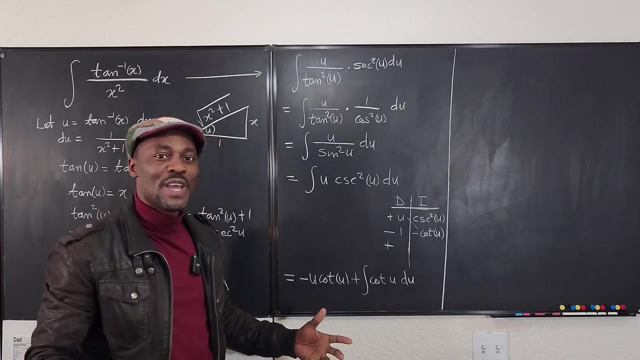 cotangent u. okay, that's part of our answer. then we're going to go this way: negative one times negative cotangent, that's going to be plus the integral of one times. this is just cotangent u du. okay. so as long as we can integrate this, we get our answer. this is the only thing left now. how do you? 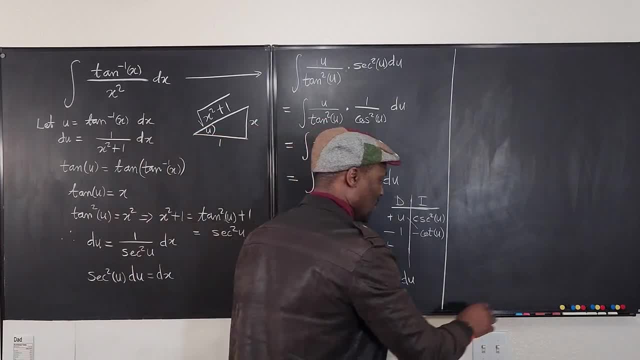 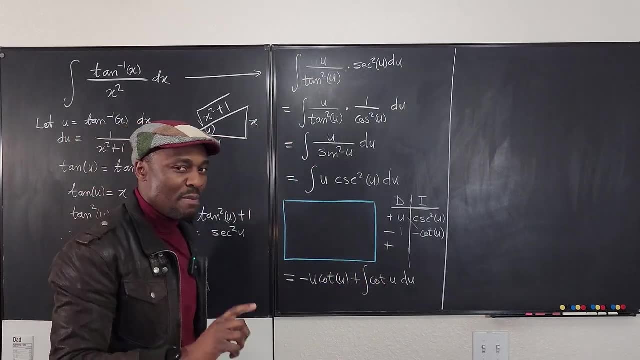 integrate cotangent u. so let's go, let's do the work here. cotangent u, let's integrate cotangent u and let's do the work here. let's do the work here. let's integrate cotangent u, tangent u here. Now, remember, cotangent is cosine over sine, So it's an easy thing If you've 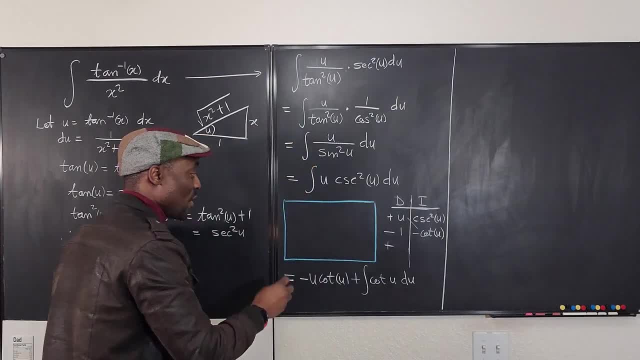 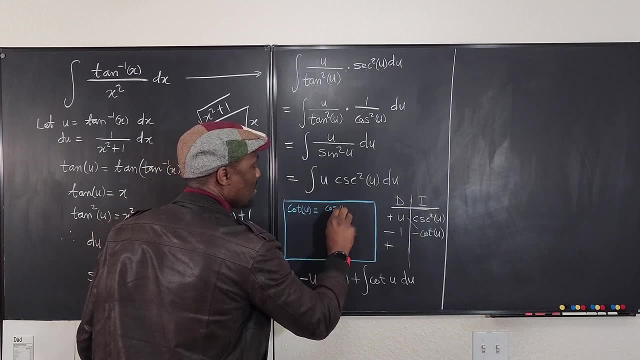 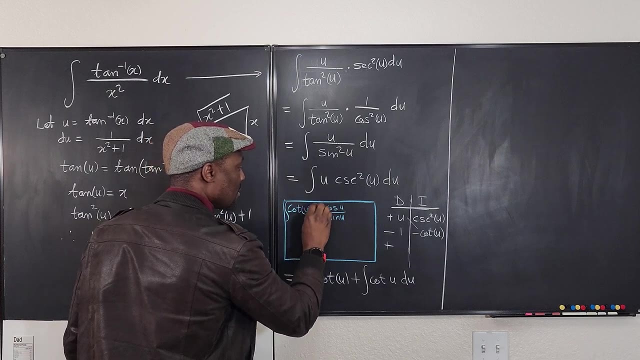 memorized it. good, If you've not memorized it, this is how you integrate cotangent. Remember that cotangent, cotangent u will be equal to cosine u over sine u. okay, So when you take the integral of this du, it's going to be the integral of cosine of u over sine u du. 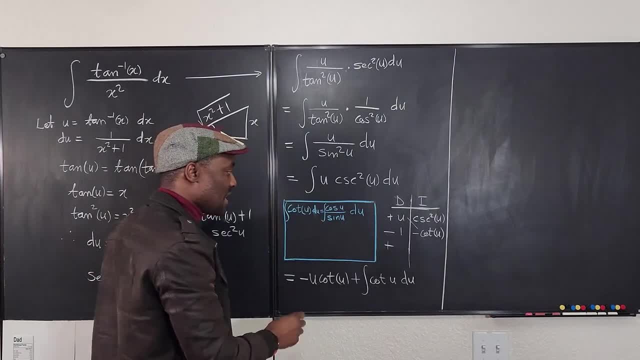 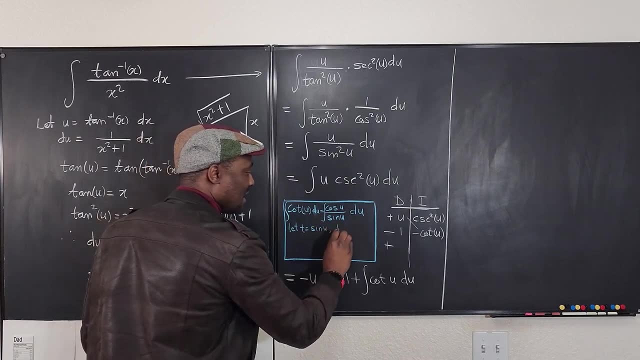 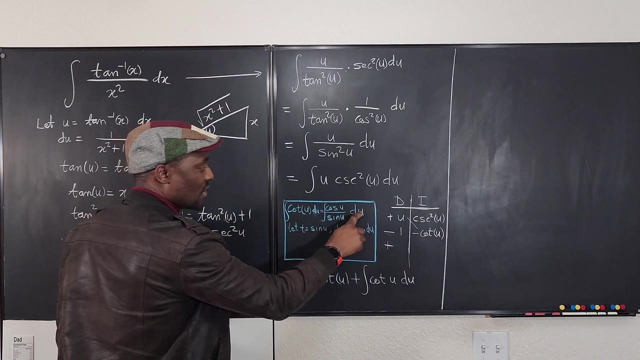 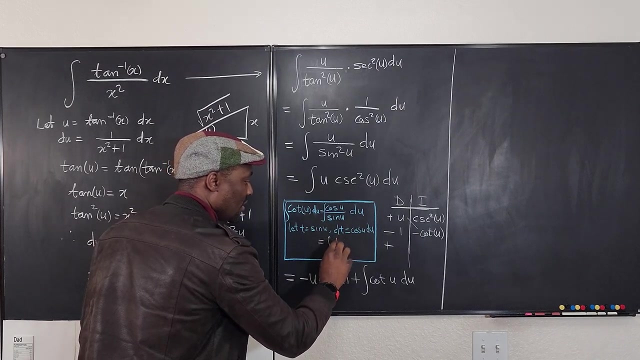 And you can now do a t substitution. You can say: let t be equal to sine u, so that dt will be equal to cosine u du, which is what's on top. So you can go back and say: this integral is equal to the integral of 1 over t. 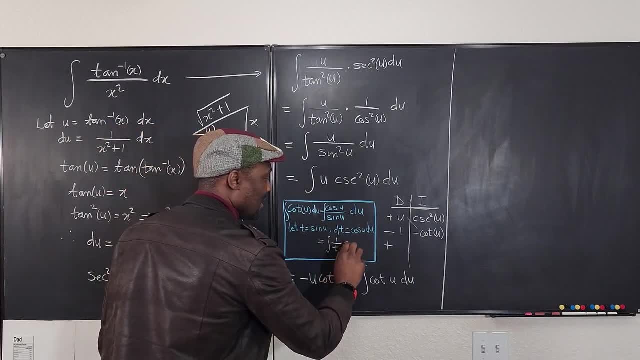 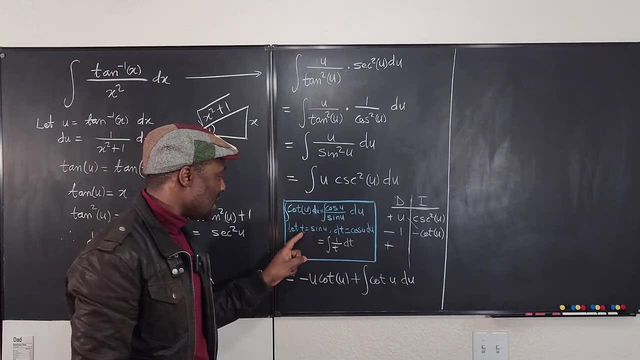 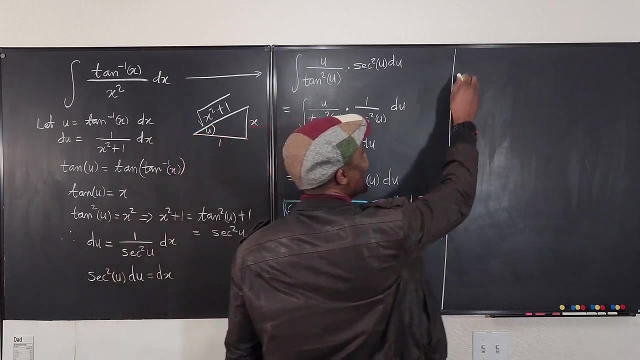 dt and what is 1 over t? dt is the natural log of t. so we know that since our t is sine u, our answer is going to be the natural log of sine u. so we're going to say that our next line. but some people have memorized this. if you don't have it memorized, let's so let's put a small. 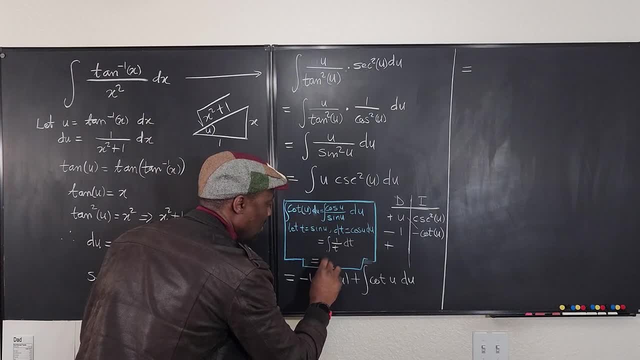 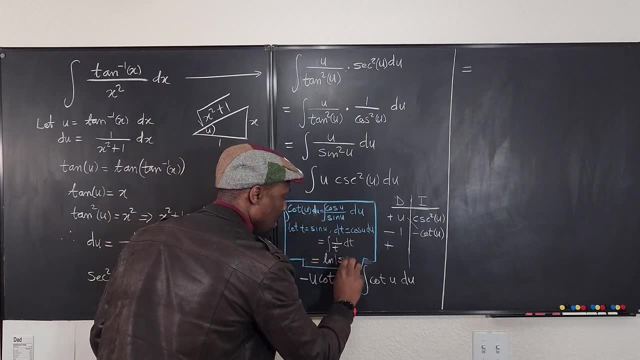 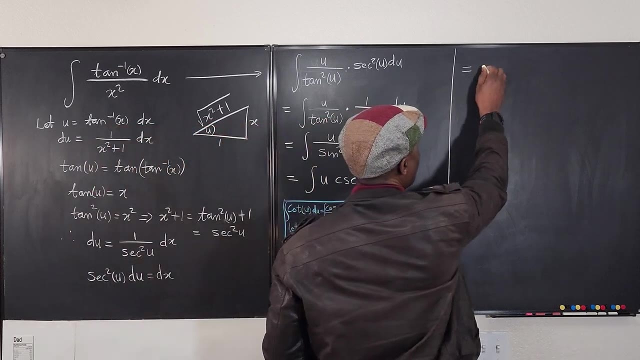 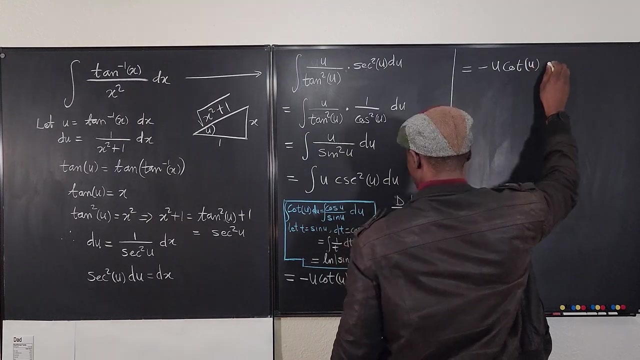 answer here. so our answer is going to be: this is equal to the natural log of t, but we said our t is sine u, that's sine u plus c. but we don't need the c yet, we just need sine u. so the answer to this is going to be negative: u multiplied by the cotangent of u. cotangent of u plus. 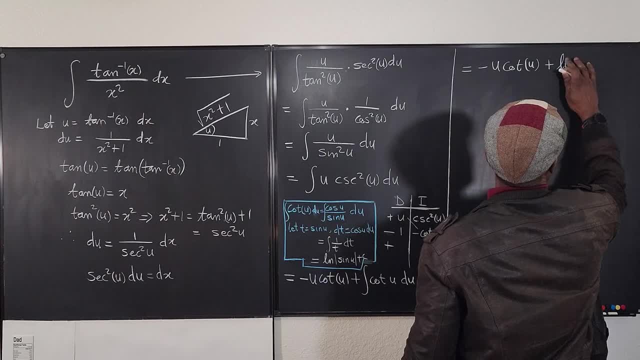 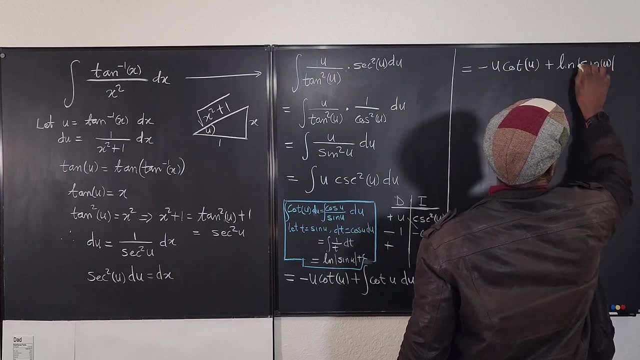 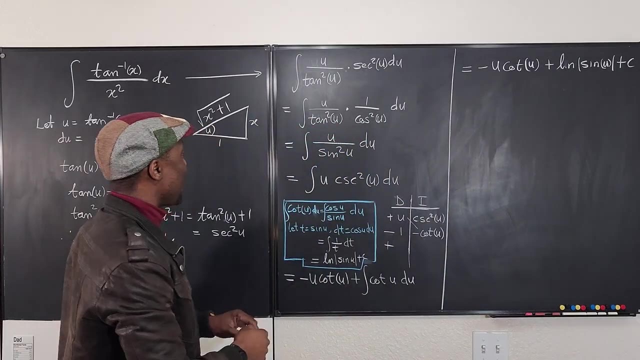 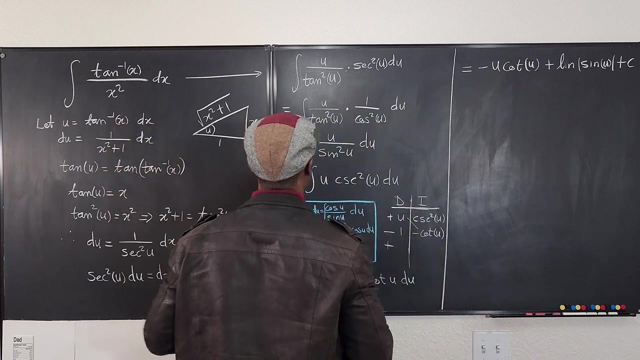 the natural log, the natural log of sine. u okay plus c. okay, that's it. we're done with the integration. we just need to go back and put back what u was. what was u? again? let's go back. u was arctan of x, u was arctan of x, so our 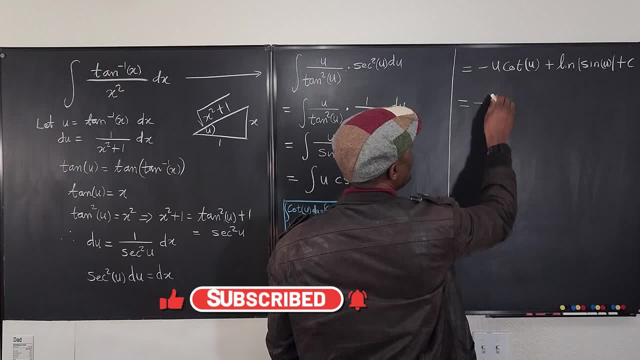 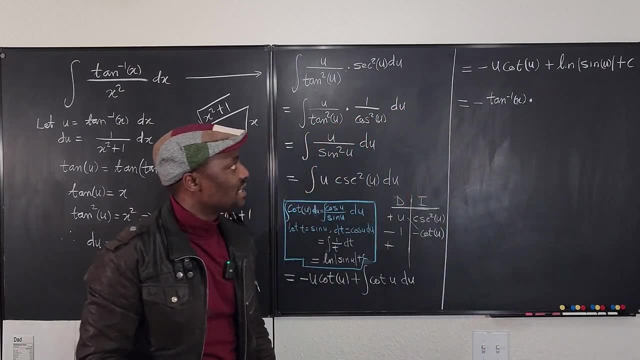 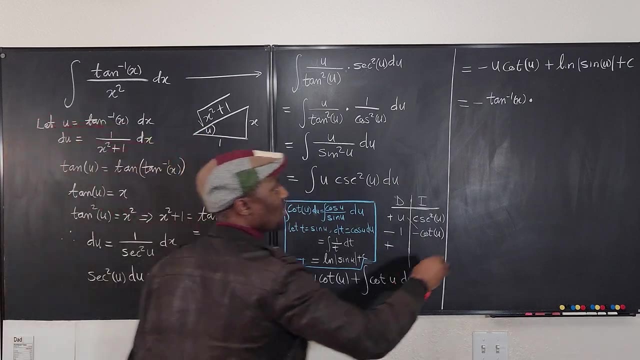 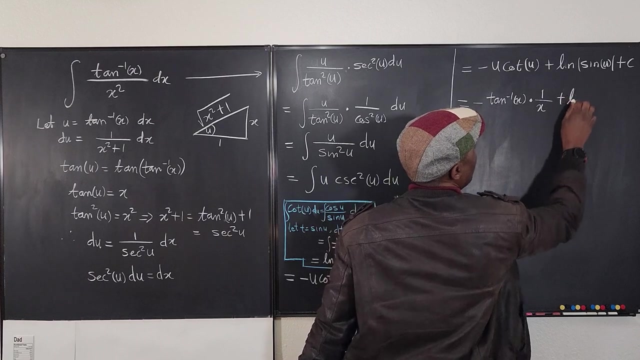 answer will be equal to negative. u is arctan of x. okay, multiplied by the cotangent of u. we'll go back here. what is cotangent? cotangent is adjacent over hypotenuse, so that's going to be one, sorry. adjacent over opposite, over x plus the natural. 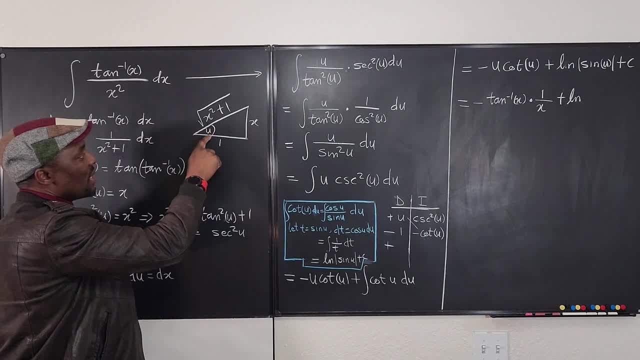 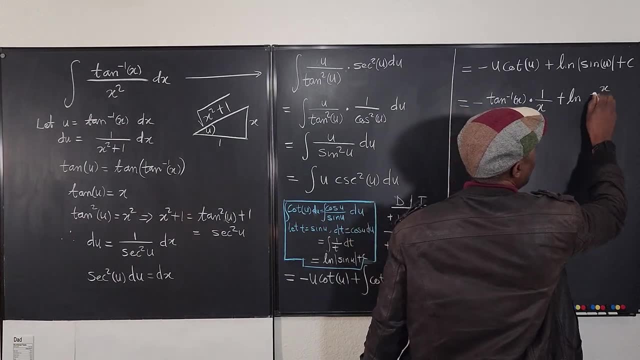 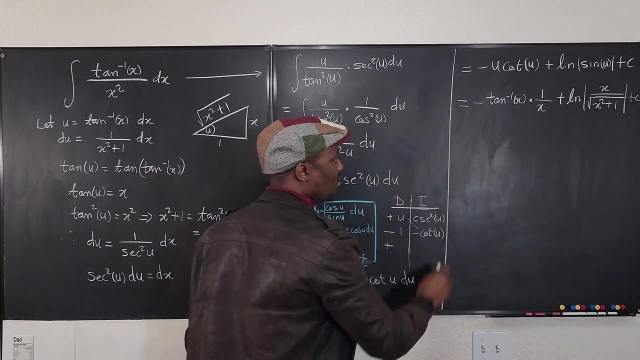 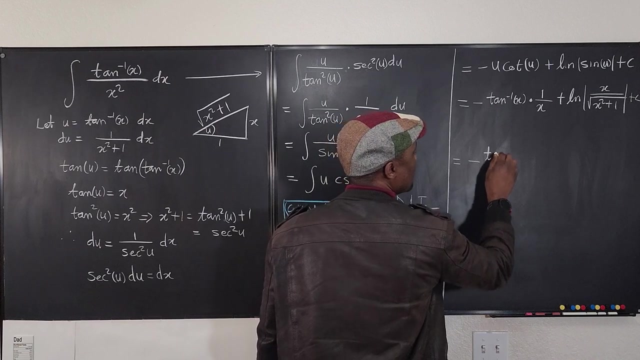 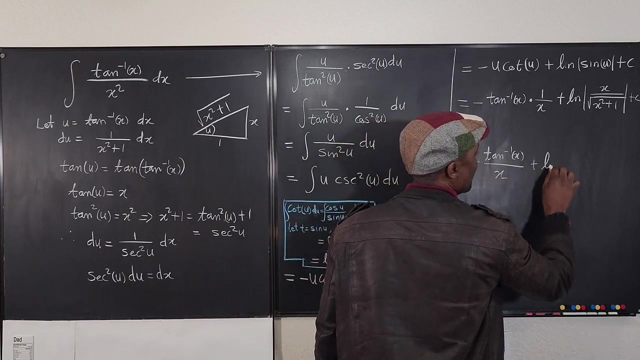 log of something which is the sine of u, what is sine u, opposite over hypotenuse, which is going to be x over the square root of x, squared plus one plus c. okay, let's write it neatly here. so this integral is: we can put this x under this, it's going to be negative arctan x over x plus the natural log. 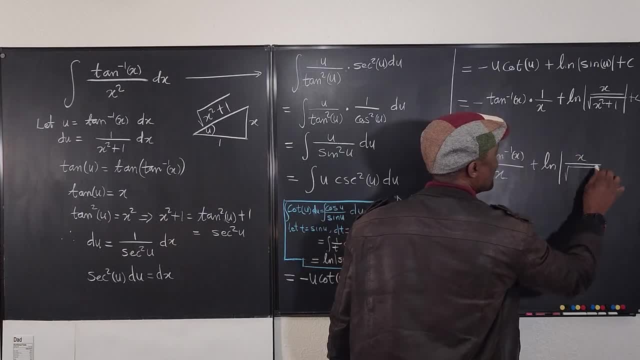 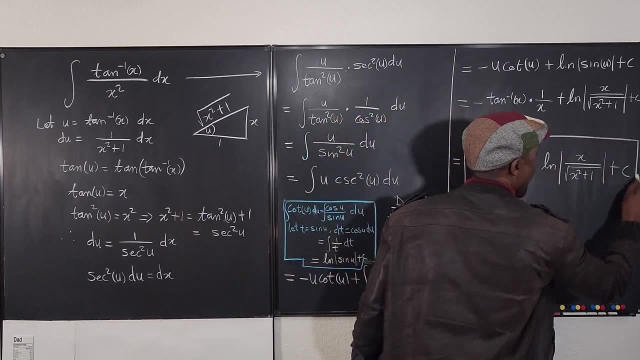 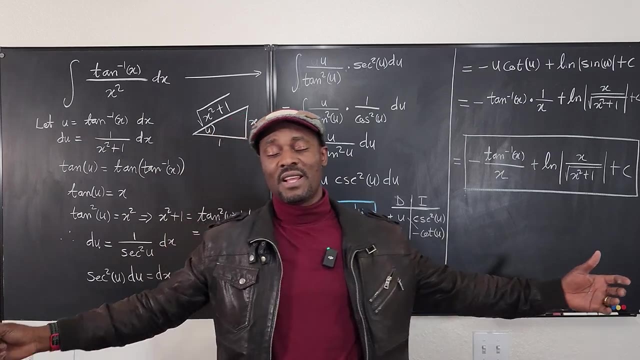 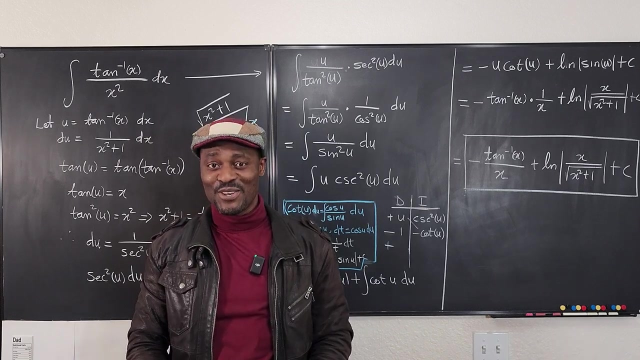 of x over the square root of x, squared plus one plus c. this is a beautiful one. i love it because it helps you do a lot of manipulation. your algebra and your trig skills return, and joy returns. hope you learned something. if you did leave a comment in the comment section, i'll see you in the next video. never stop learning. because those who stop learning have stopped living bye.